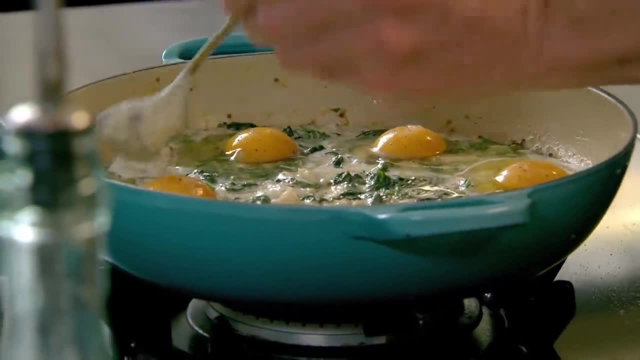 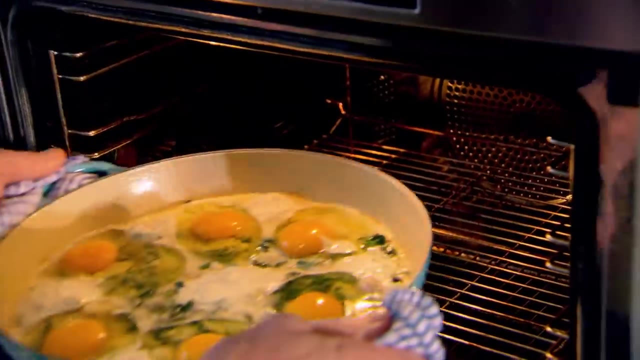 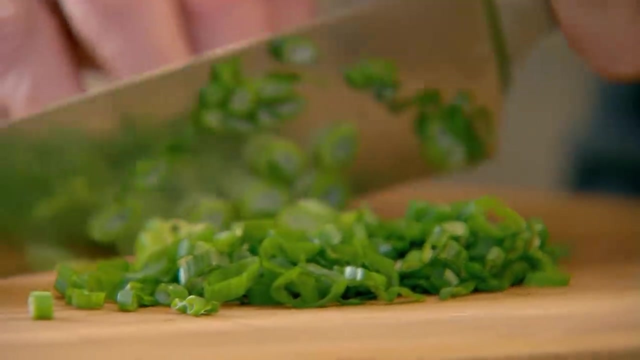 Get the remainder of your creme fraiche and put a little dollop in between- That adds richness to the egg whites- Into the oven at 180 for 10 to 12 minutes. Whilst the haddock and eggs bake together, I can knock up a simple spring onion garnish. 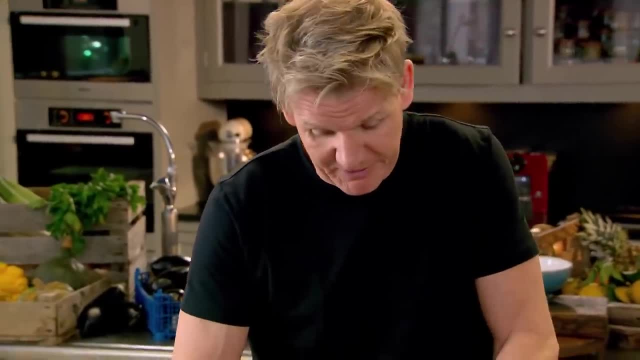 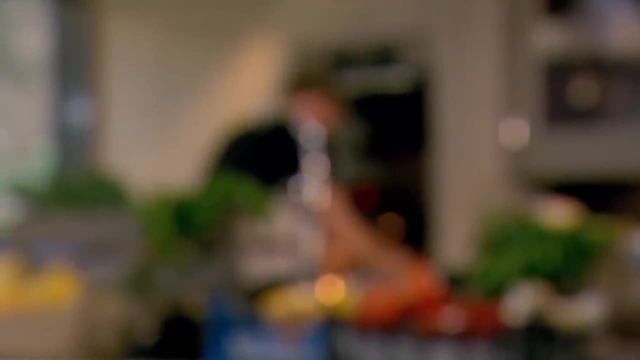 And professional kitchen chefs refuse to use the top of their spring onions. but I love that nice dark green flavor. It's less harsh than the white. The smell of baked mustard You can't beat. That is beautiful. Spinach is almost melted. 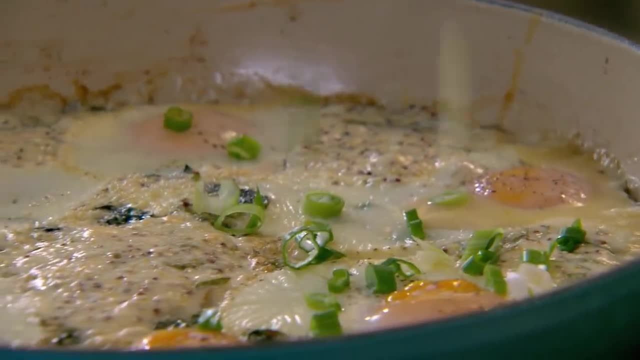 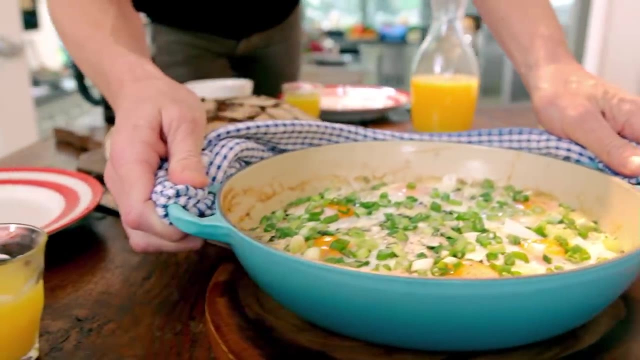 in with the haddock. Now just sprinkle your spring onions. That gives that really nice sharpness. Wow, My ultimate hearty breakfast: smoked haddock and spinach-baked eggs So packed with protein and iron you'll be raring to dive into the day ahead. 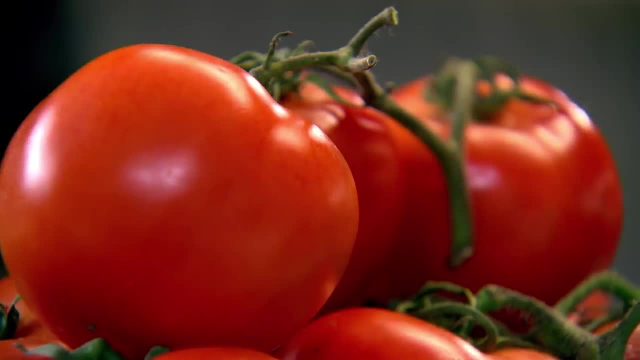 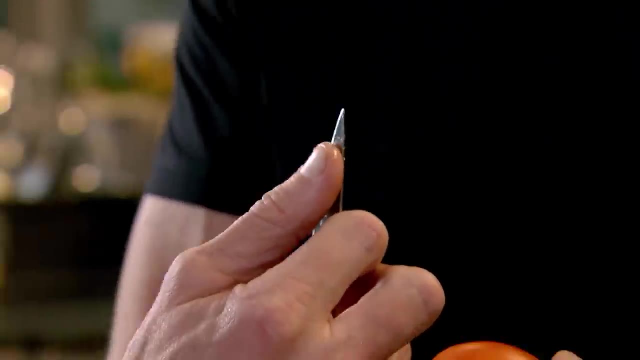 Roasted tomato soup. Beautiful vine tomatoes. The riper the tomatoes, the better the soup. Take the core out, Get your thumb and place it half a centimetre underneath the tip of your knife. Place it in and then just twist around. 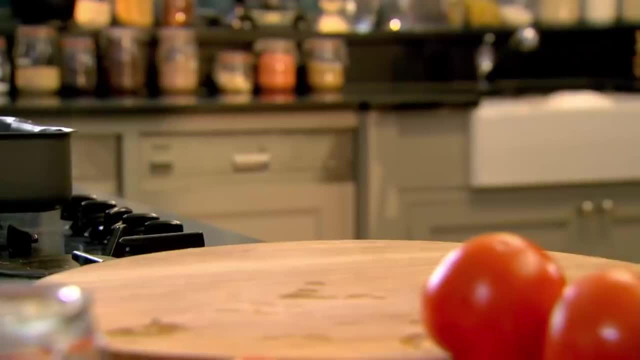 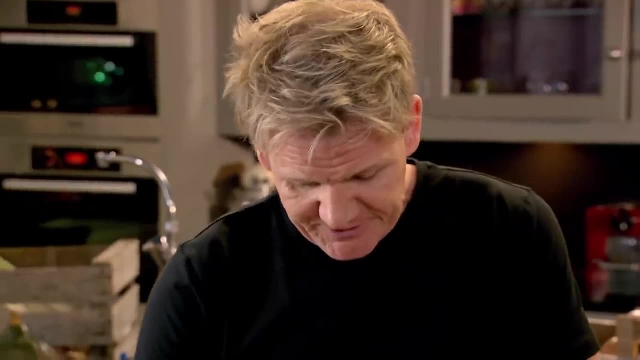 That's the only part of the tomato that we're not using: Red onion and garlic. Red onion because it's sweeter than a white onion. Slice your onions and your garlic Nice and fine. Traditionally, we make it in a pot. 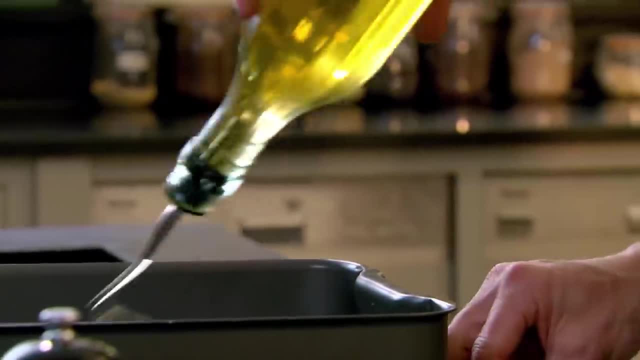 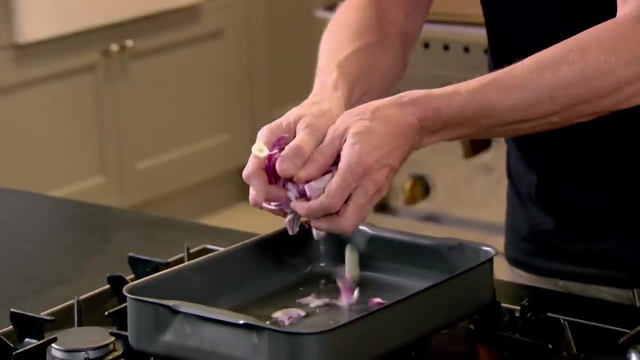 It's so much better to start it off on top of the stove, searing the tomatoes and the garlic. When it goes in the oven, you actually roast the tomatoes and they don't stew. There's a big difference in flavour. Be quite generous with the olive oil. 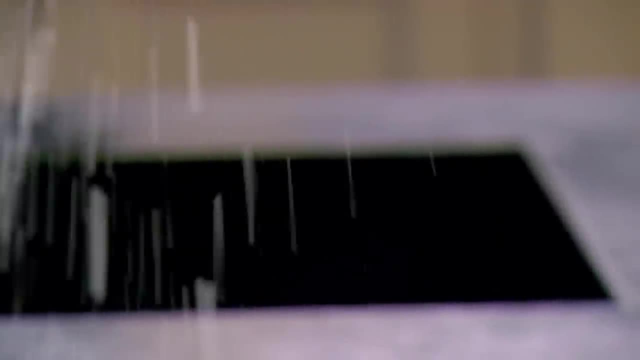 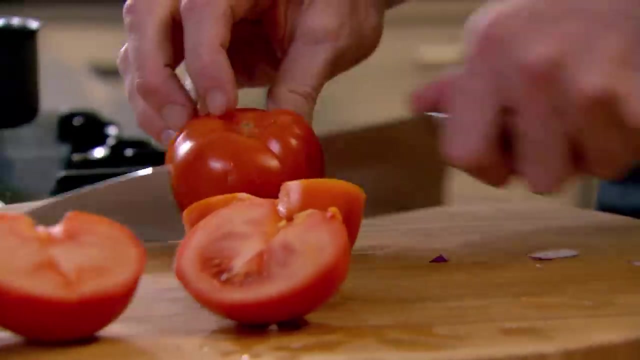 It makes the soup nice and glossy. Shiny salt pepper and then a little teaspoon of cayenne just gives it that heat, but it's not as fierce as chilli. Take your tomatoes and just slice them in half, and then a little touch of sugar. 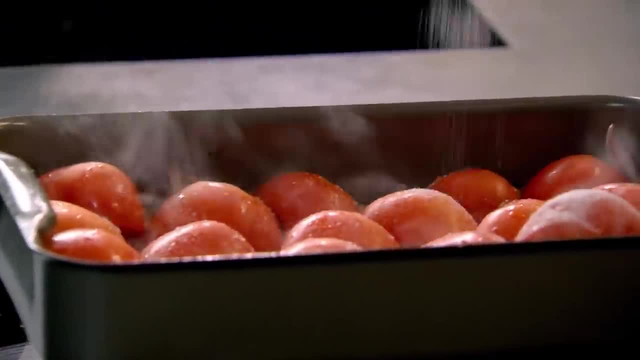 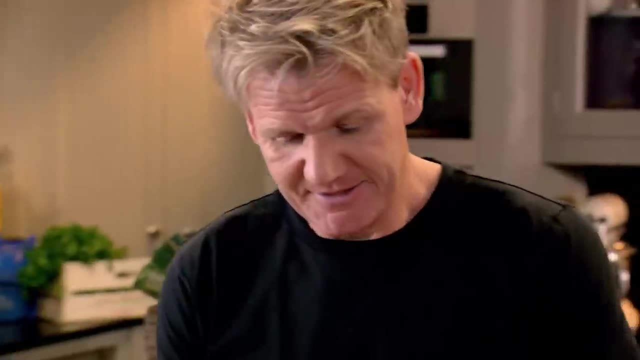 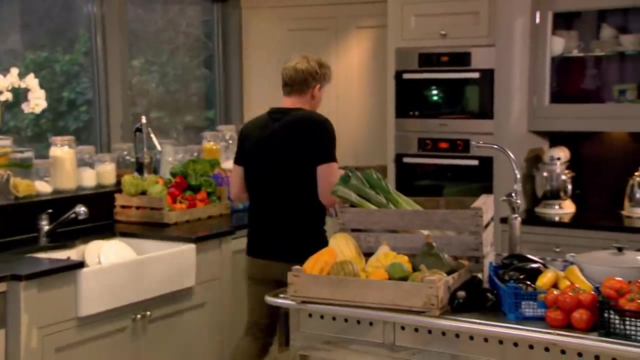 That's going to help intensify the sweetness. A little sprinkle of aged balsamic vinegar gives that nice, dark, rich acidity to the soup. Into the oven: 20,, 25 minutes, 180.. To make my soup even more irresistible, I'm going to make a punchy sun-dried tomato pesto to drizzle over the top. 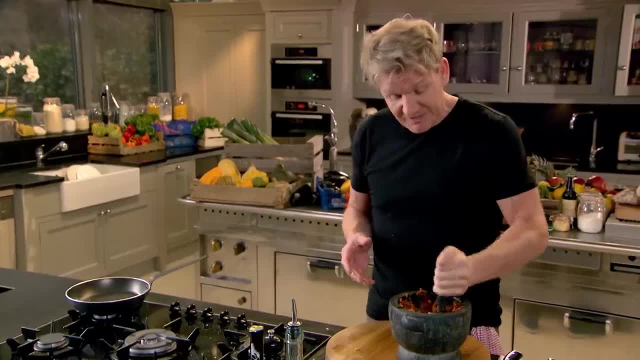 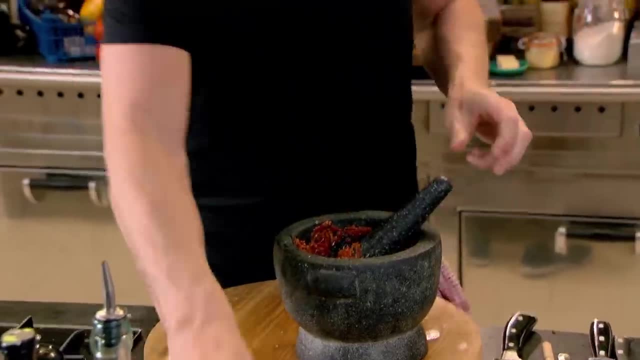 Now I'm making this in a pestle and mortar because you feel so much more in control And you're not depending on a blade that's whizzing around at a thousand miles an hour. Next, in a dry pan, toast off some pine nuts. 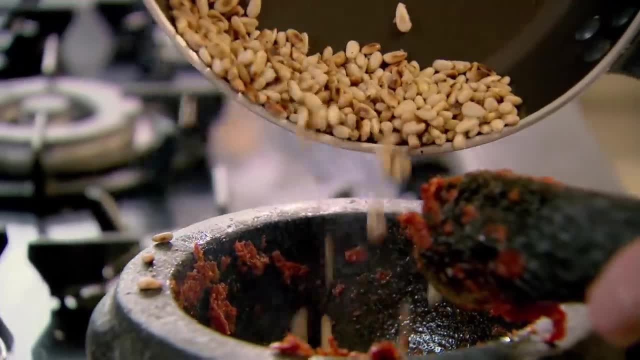 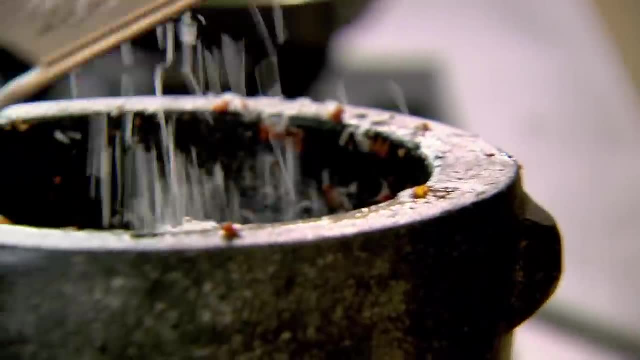 Toast them to the absolute max and then, in The smell in there is incredible Parmesan, Lightly grate that. This is where it starts to become creamy. Extra virgin olive oil Doesn't need salt, because the parmesan's going to season it for you. 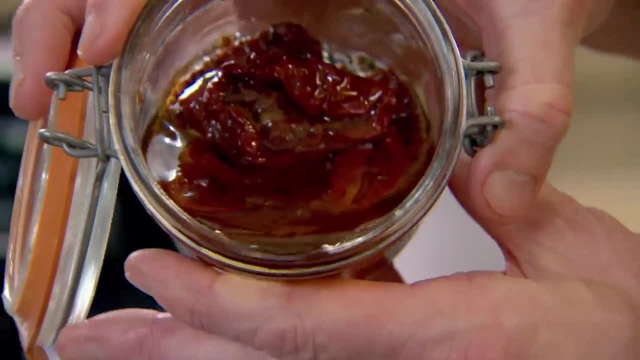 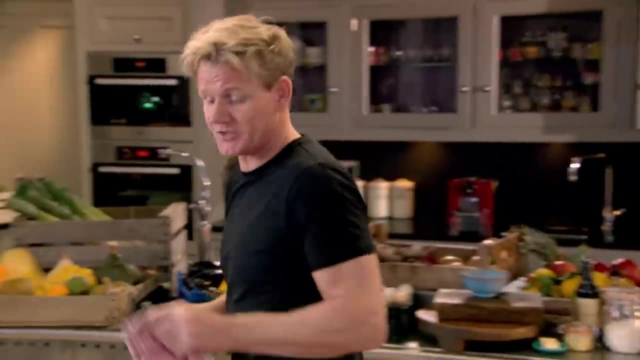 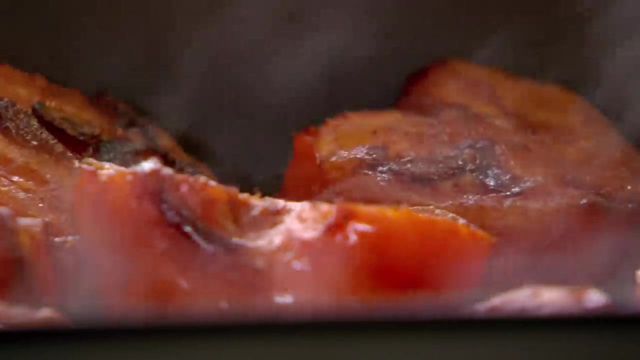 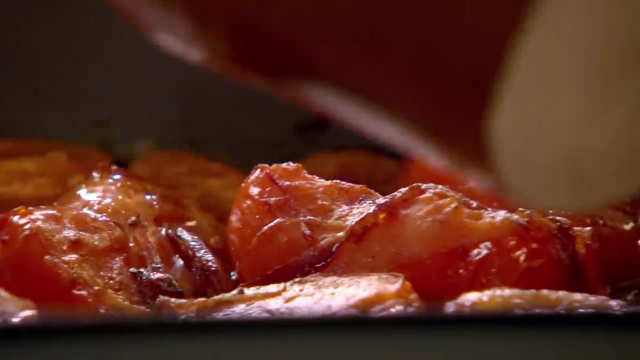 And just take a couple of tablespoons of the oil of the sun-dried tomatoes we're in Really helps to make that stunning pesto. I can smell those roasted tomatoes. Want them out, Wow, Wow. Next, pour in a little vegetable stock or chicken stock so it sits halfway up the tomatoes. 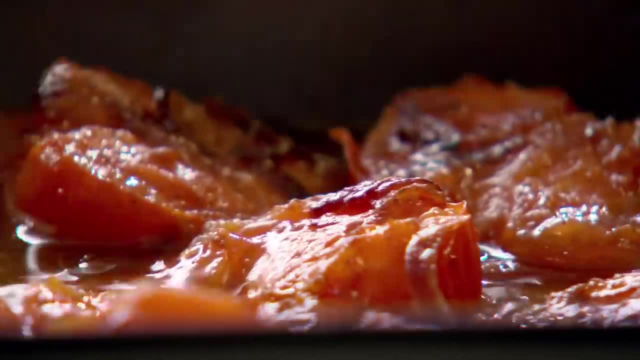 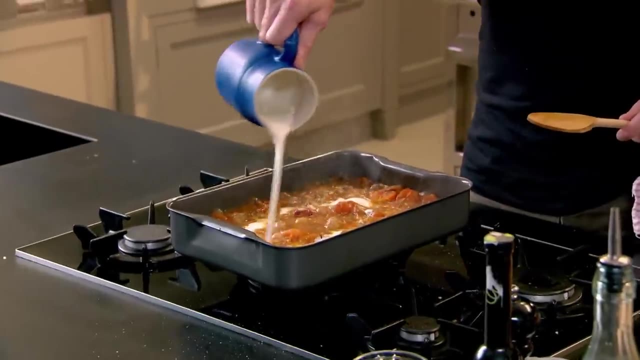 Put your spoon through those tomatoes, They break up instantly. Bring that up to the boil. Let it simmer for three or four minutes. I want to make it a little bit more creamy now. Cream in, Give that a little stir. You can keep it rustic and get your masher in. 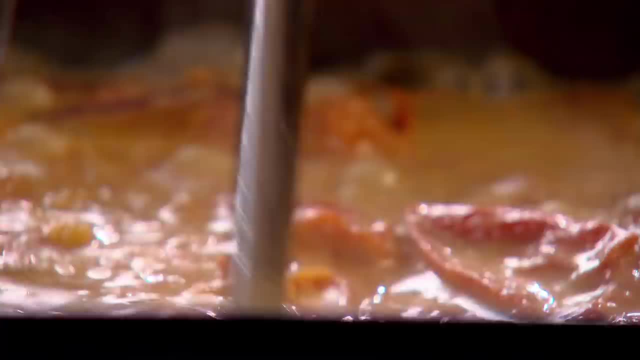 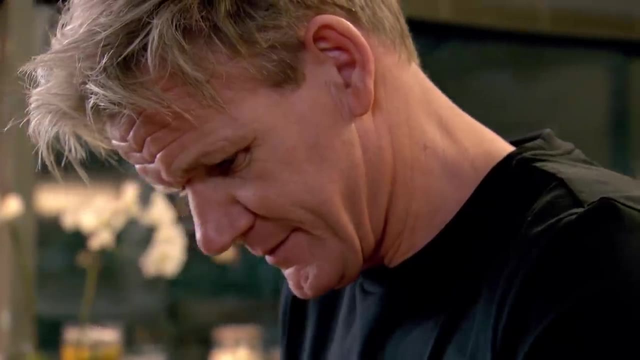 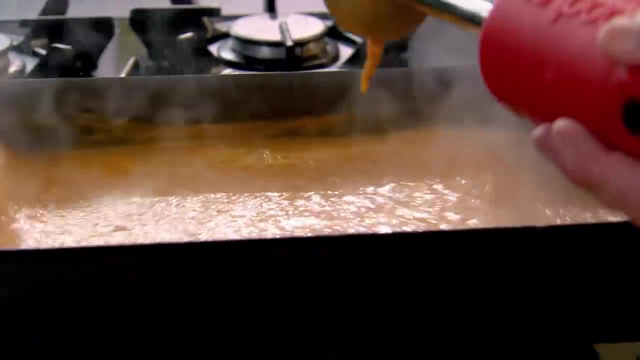 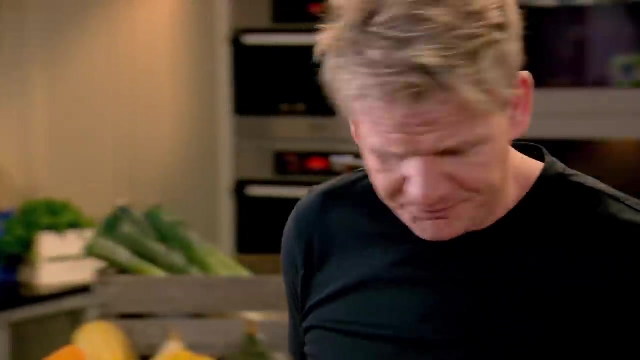 And you've got that nice, thick, rich, chunky tomato soup. Or get yourself a stick blender Blitzing it like that You deglaze the bottom of the pan and you get all those amazing flavors from the bottom. That's delicious. 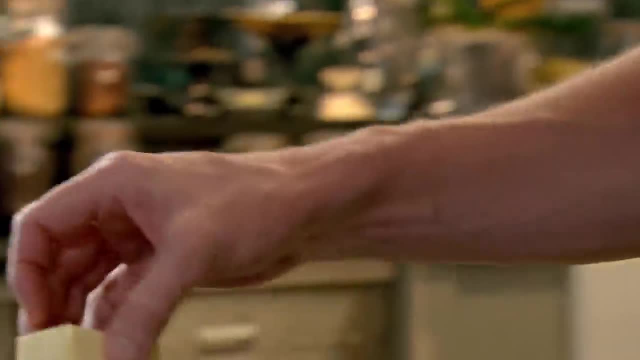 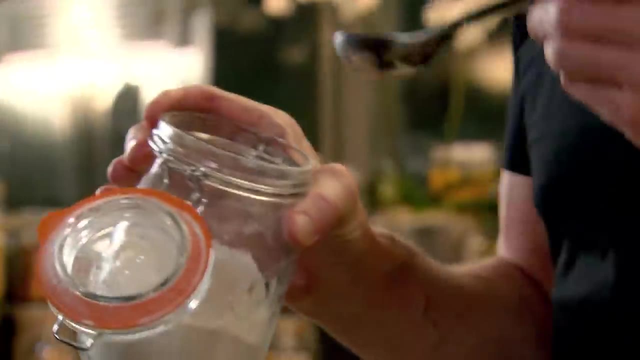 To make my lunch extra hearty, I'm going to knock up a deliciously gutsy version of cheese on toast to go with my tomato soup- Bosh rabbit- An absolute classic. I'm going to make a roux: 50 grams of butter, three nice tablespoons of flour. 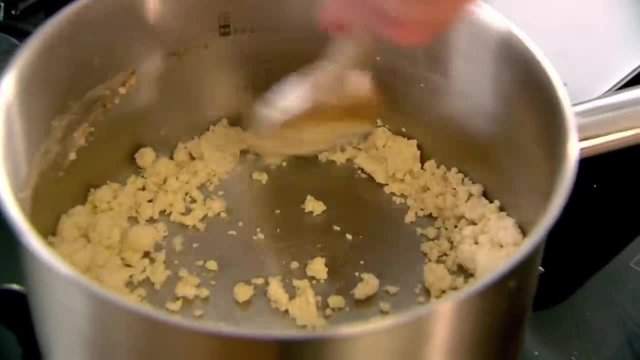 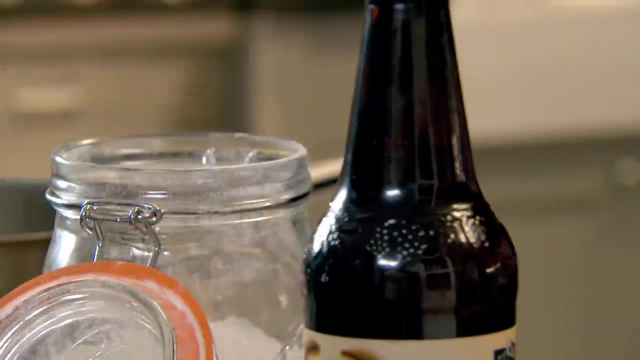 And that's all a roux is basically. Traditionally you would use flour, butter and milk, But in Welsh rarebit the milk is often cheekily substituted for a stiff slug of stout. It gives it that strong, gutsy flavor. 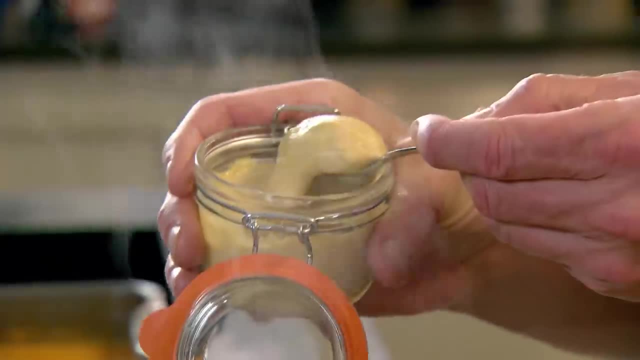 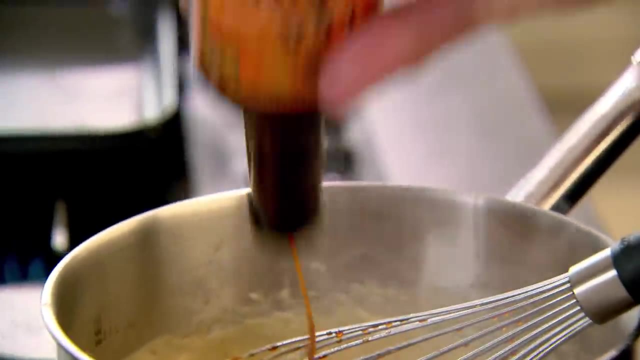 I want it nice and thick. Make sure those lumps are out, A nice teaspoon of Dijon mustard And then season it Nice and spicy, And then that superavantagious source gives it that delicious, intriguing flavor. Now that smells amazing. 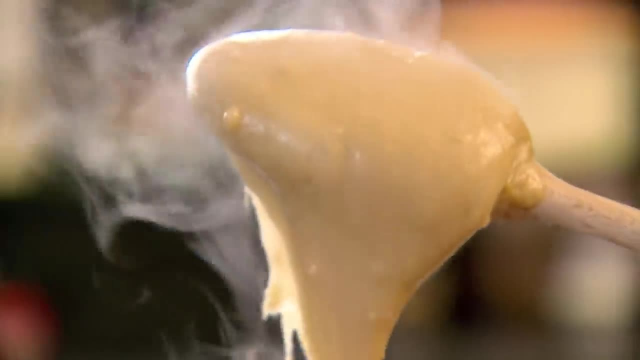 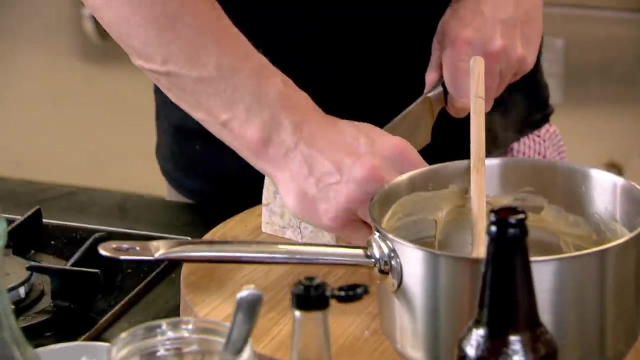 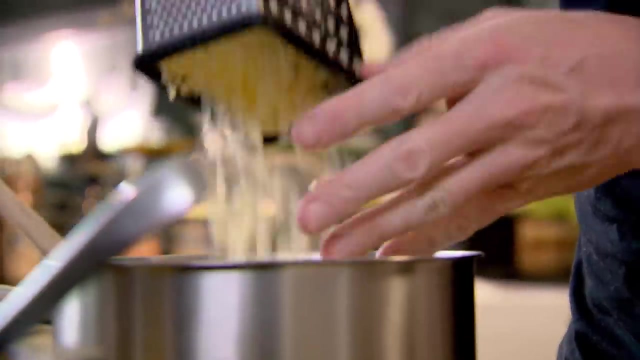 Almost brings tears to your eyes. Beautiful. Now Welsh rarebit wouldn't be a stunning Welsh rarebit without rich mature cheese soap and a great Montgomery cheddar. Goes well with beer And drop that in. Really important to put this in while the roux is still nice and hot because the cheese melts. 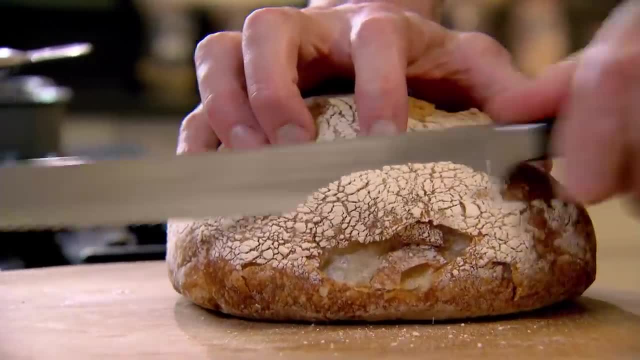 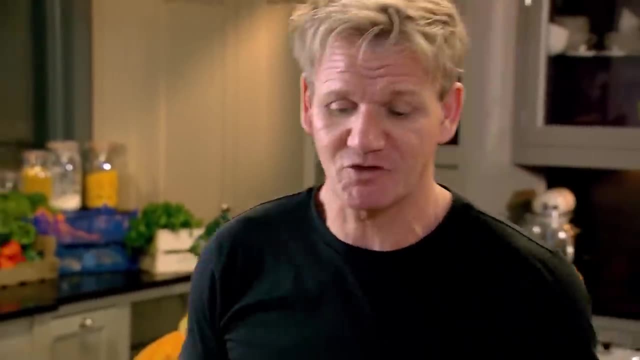 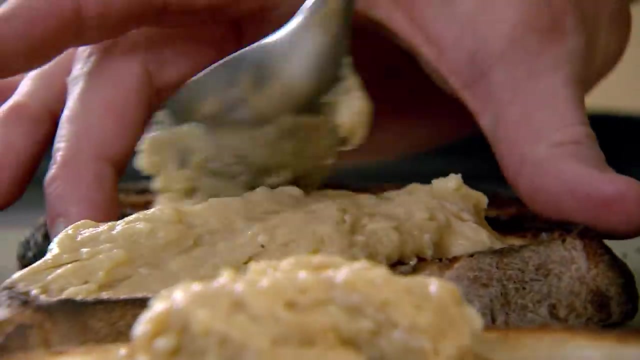 Now our spice. Now for the bread. I prefer a good rustic country loaf that will stand up to my hardcore topping. I want that nice crisp base to my Welsh rabbit. so toast it both sides. Spread that beautiful cheesy, beery, spicy mixture. 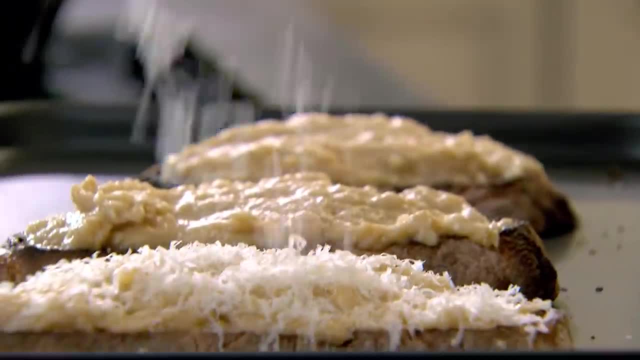 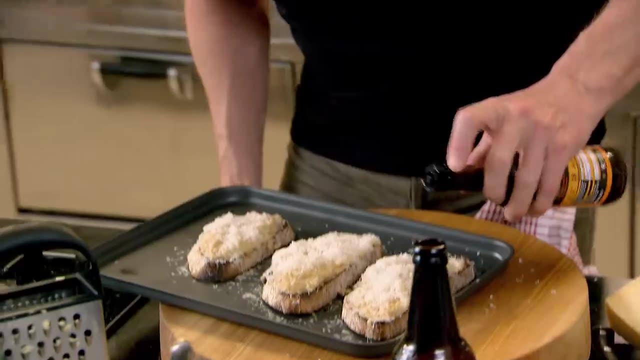 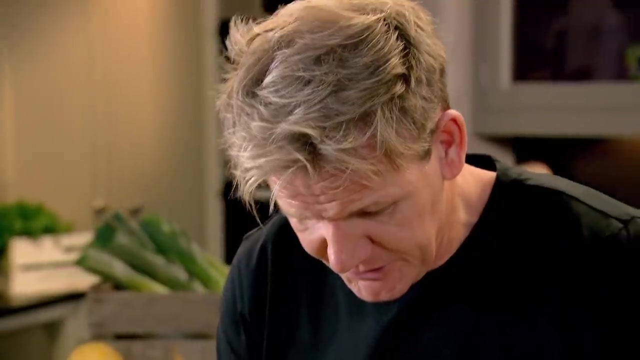 Just great. Got to blister and bubble and gratinate. God Got a little splash And back under the grill for 90 seconds In One delicious creamy roasted tomato soup. It's coming back to me all those days I had off school. 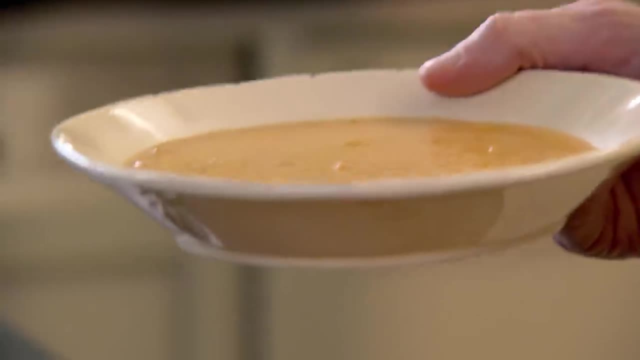 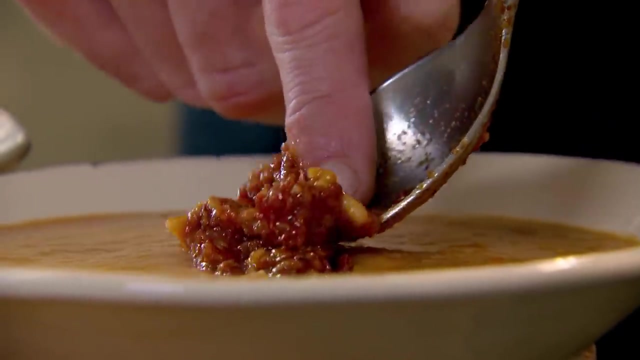 I used to purposely lie about feeling ill just to get a bowl of my mother's tomato soup. How bad was that, But my God, it was worth it. Oh, Now my Welsh rabbit Mm. Look at those babies. 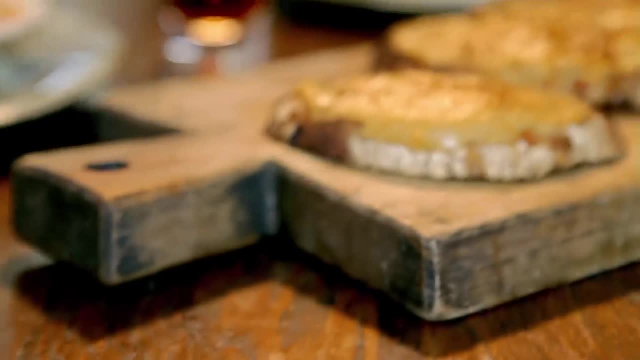 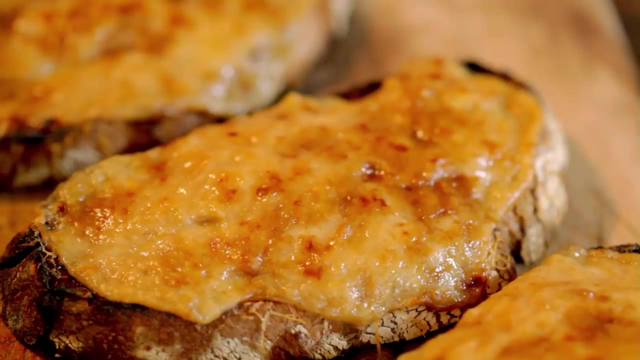 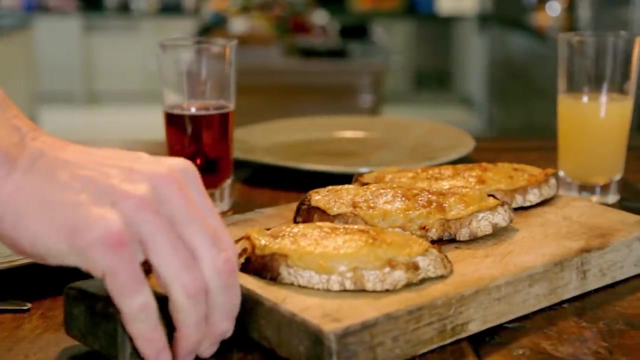 That just takes cheese on toast to another level. Wow, Roasted creamy tomato soup with a sun-dried tomato pesto, served with the most amazing, delicious Welsh rabbit. I feel like ringing in sick Beef and ale with mustard dumplings. 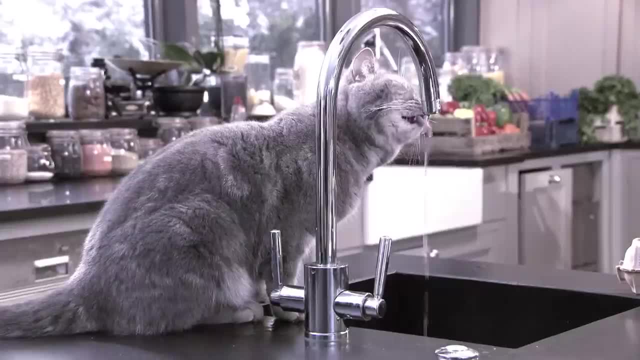 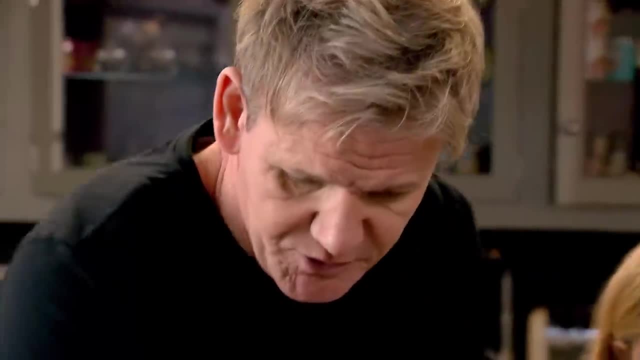 And helping in the kitchen is my youngest Tilly. Tilly, First thing. first, I'd like you to season the stew and steak A nice spoon of flour Mix. Yeah, Good girl, What's the flour going to do Dad? 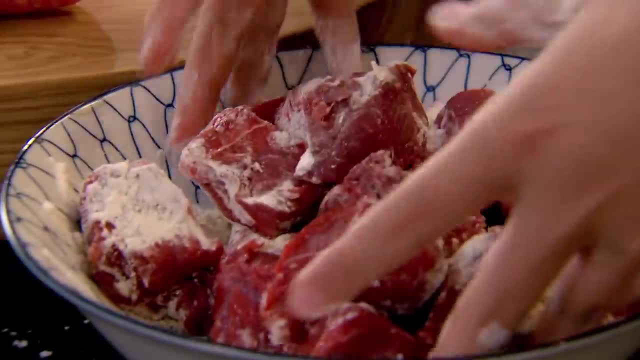 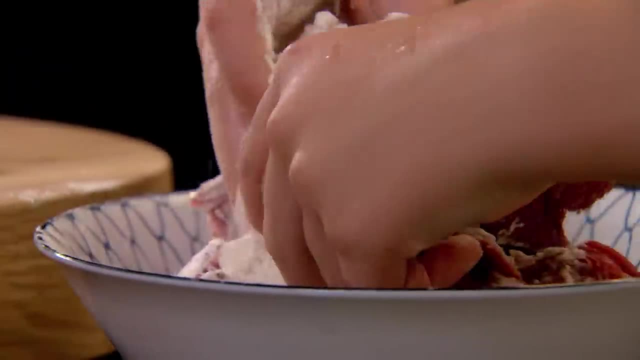 The flour helps to brown the beef. Our seasoned flour will also help to add flavor and thicken the stew. I feel a bit like a kid. that's a bit older than me, I don't know. I'm gonna try it. There you go. 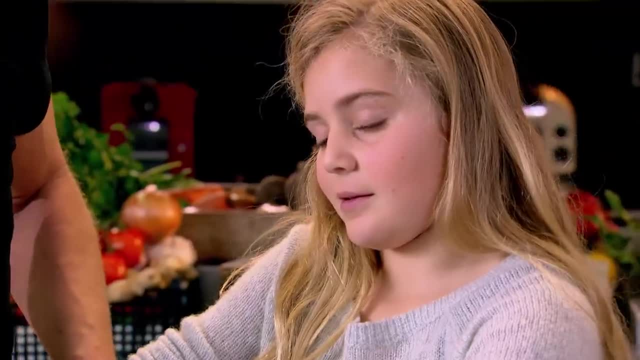 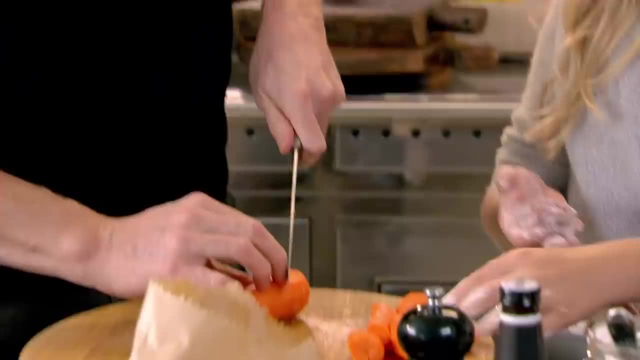 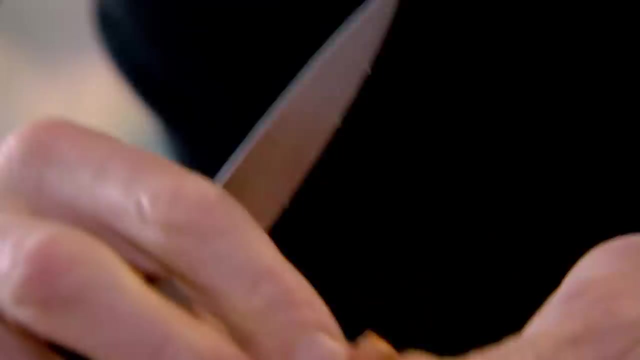 There you go, There you go, bit like marshmallows. look at the size of the chunks of the beef and I cut my carrots. literally be similar, similar size, that's right. does that mean they'll cook equally? that's right. now, these little pearl onions I'm gonna put them. 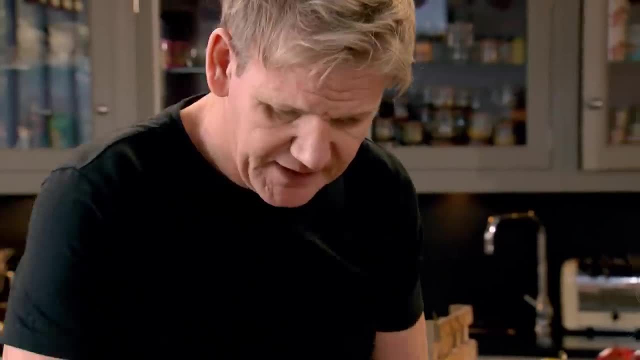 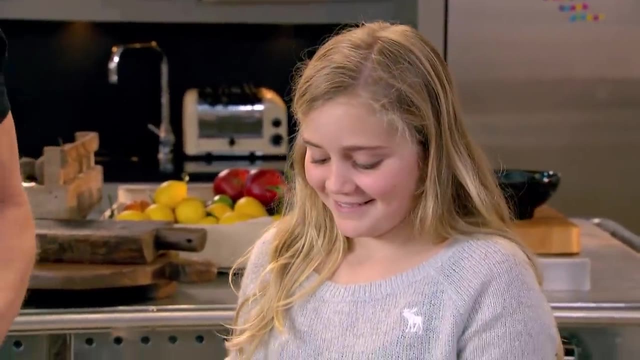 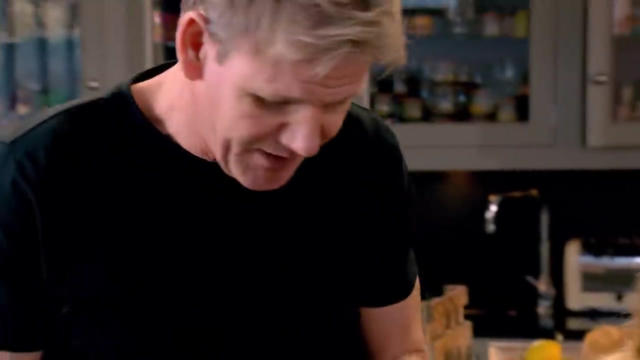 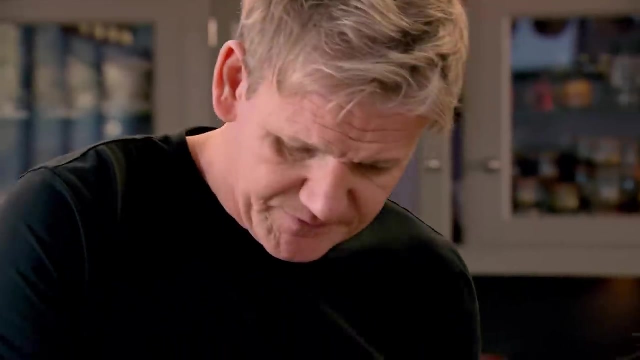 in whole as well. everything has to stay the same, otherwise it could burn. oh, we seen burn garlic before. oh, Matilda, she promised you. I'm gonna mention that. what is that? time, time and what they? babies, babies, good girl. tablespoon of oil in the beef goes in first. okay, 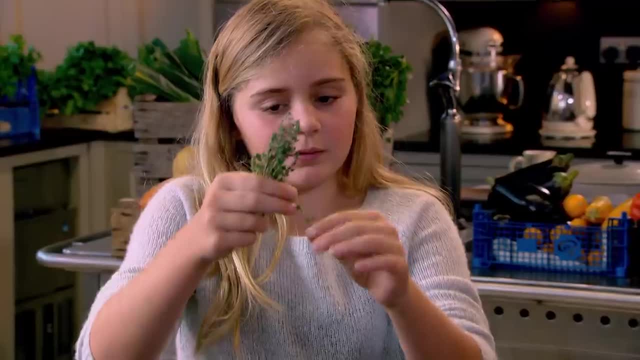 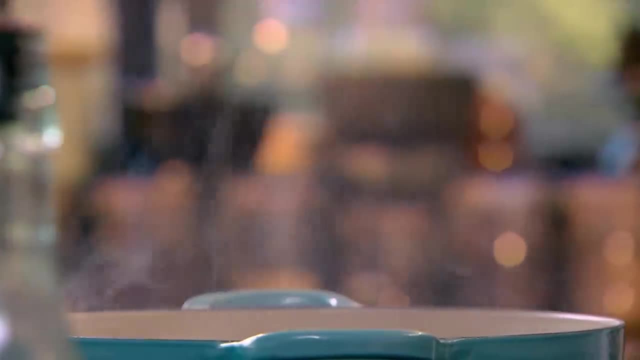 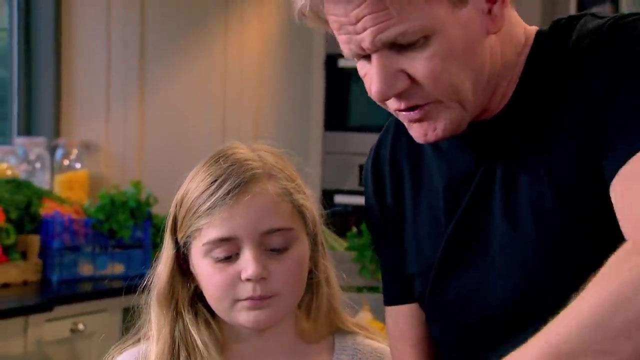 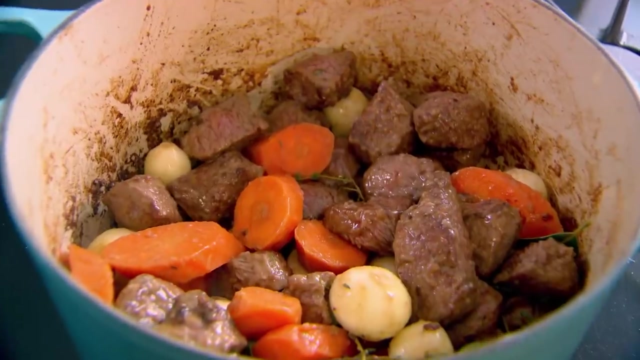 beautiful color. remember the carrots time in good girl, garlic, pearl onions in. oh good, you got a really good mix-up, mmm. are stews easy to make? daddy, stews are very easy to make, providing at the beginning you give it a little bit of love. now that's all beautifully browned. mmm, that is beer and that's gonna. 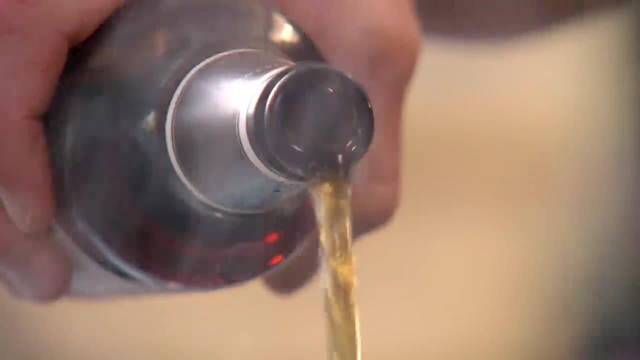 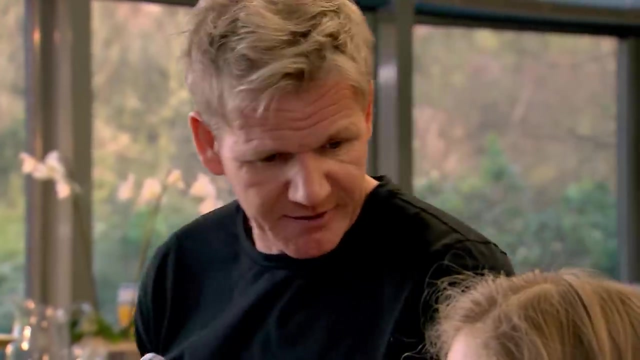 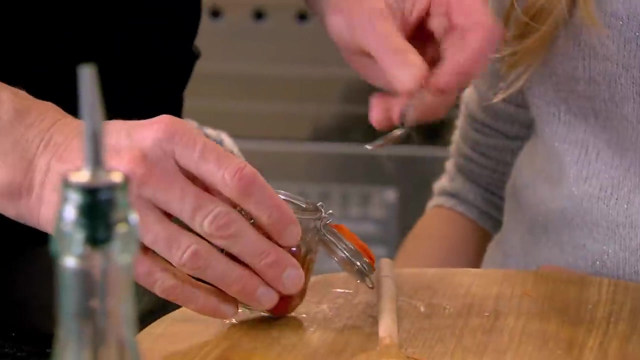 deglaze the pan. adding beer or stout helps to tenderize the beef and give it a hearty, delicious flavor, and that's the only way I want you to taste beer in a stew. yeah, I want to add in a couple of teaspoons of tomato puree please, in fact, three please, cuz it's so. 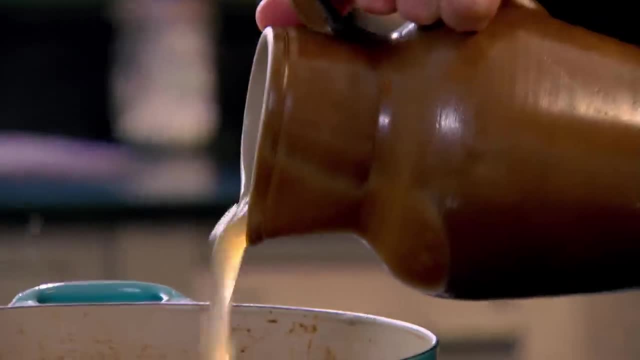 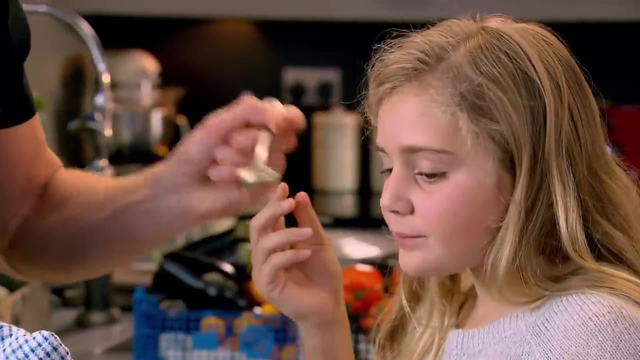 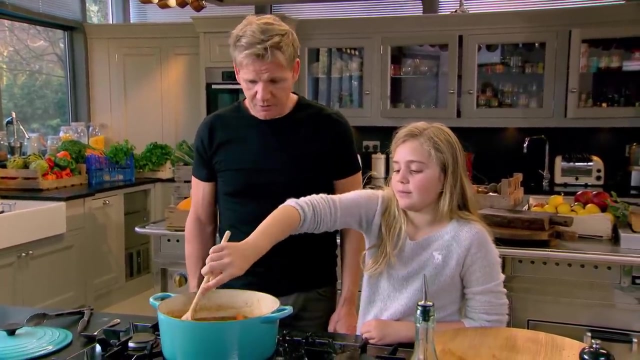 nice. there's one final thing in there: cover the stew and steak with a beef stock. give that a little mix with daddy, please. Wow, that's really nice. it's not even cooked yet. do you keep all these veggies ready now- Yes, vegetables in when you serve it to people. 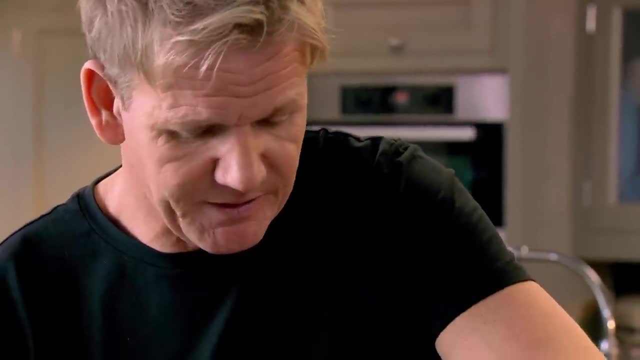 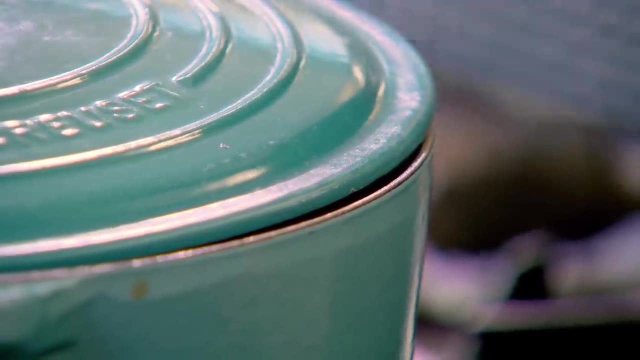 Oh yes, Is the garlic going to be burnt? Excuse me, Right, and we always put the lid with a little bit, Just a little bit, so it can breathe. That's right, and not make the stew all watery. 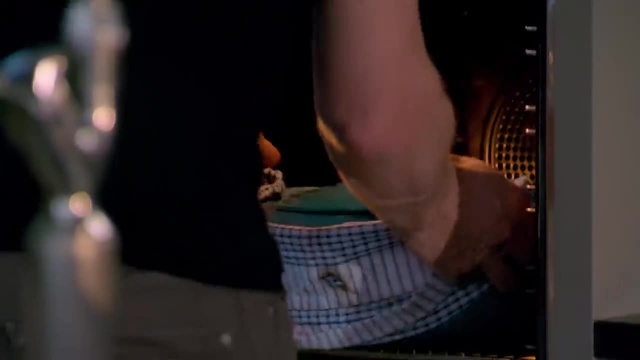 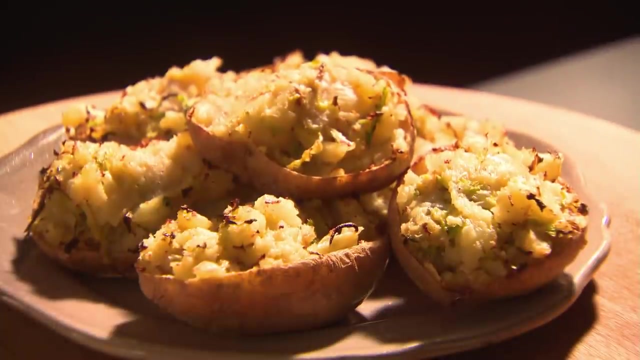 Into the oven at 150, please Tills for about 2 and 1 half hours And now you can focus on your homework. Fun Time to knock up two delicious hearty potato classics in one Twice-baked bubble-and-squeak jacket potatoes. 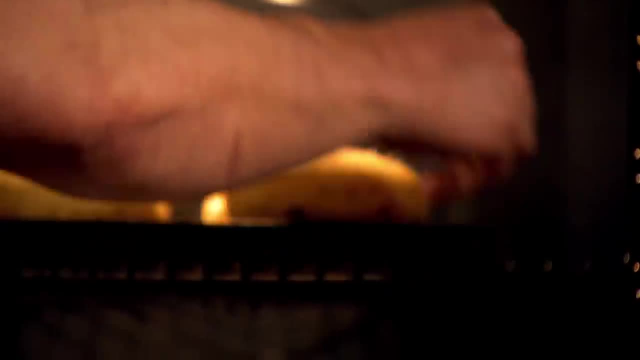 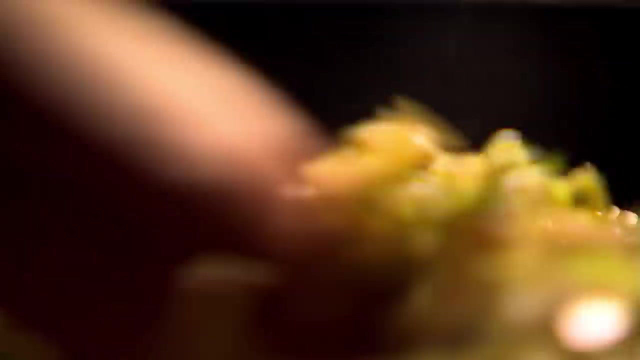 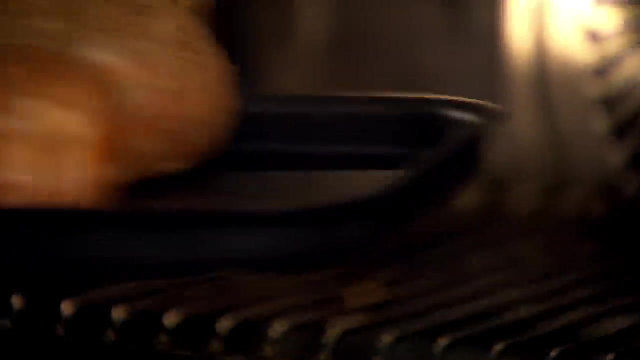 Start by baking large potatoes in a preheated oven at 180 degrees. Shred 1 third of your savoy cabbage and saute in butter and add a dash of water until tender. After about half an hour your potatoes should be crisp on the outside and cooked. 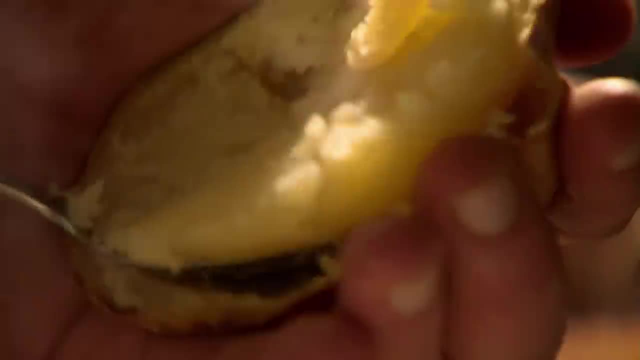 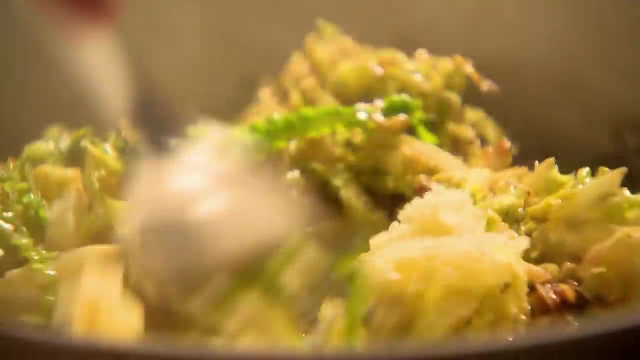 through in the middle. Slice them in half and scoop out the soft potato center. Then mash with a couple of knobs of butter, mix in the cabbage and season to taste. Spoon this mixture back into your potato shells and into the oven for a further 10 minutes. 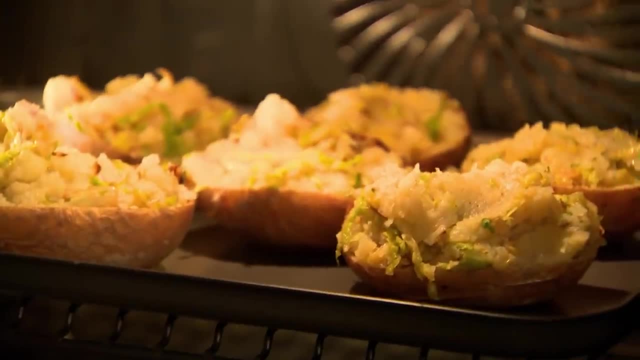 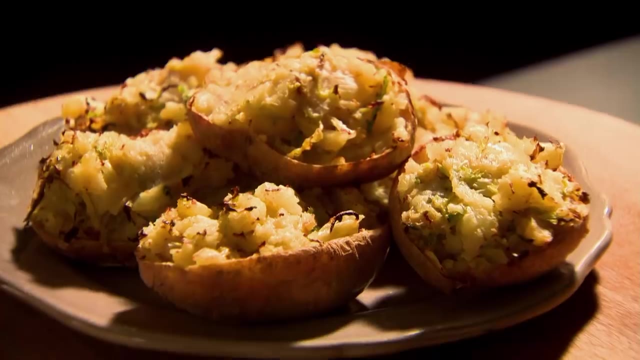 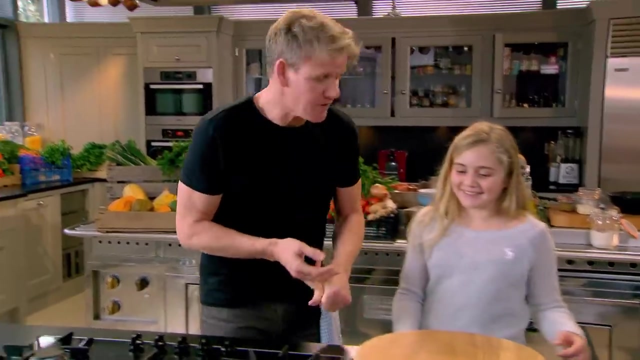 or until the tops are nice and crispy and golden. Two delicious hearty potato classics in one Twice-baked bubble-and-squeak jacket potatoes. Right, homework done. Yep, Beef stew is stewing, Stewing. Let's get on with our delicious hearty. 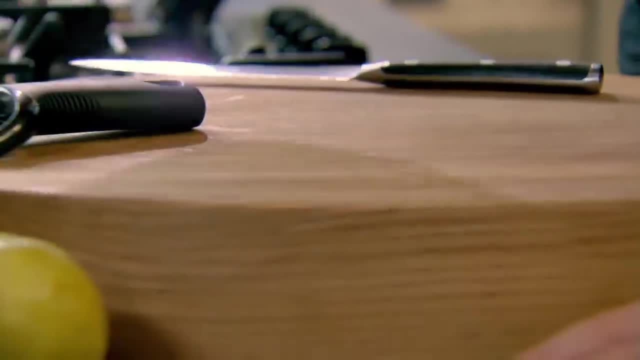 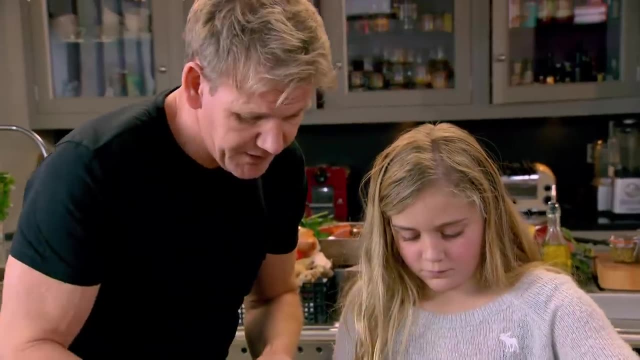 pear tart. I've been looking forward to this. You and I, chef, are going to prep the pears. So if you peel our top and tail into quarters, pears go soft in the oven very, very quickly. So if we're going to put them on a tart, 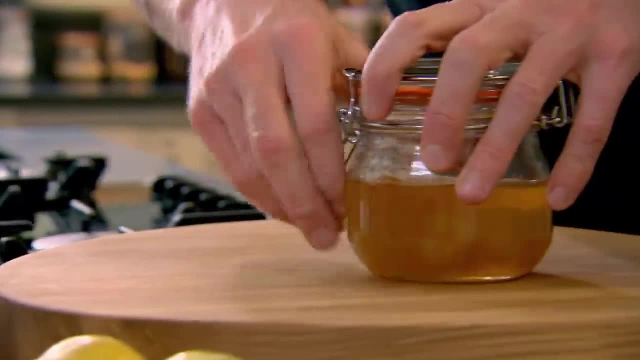 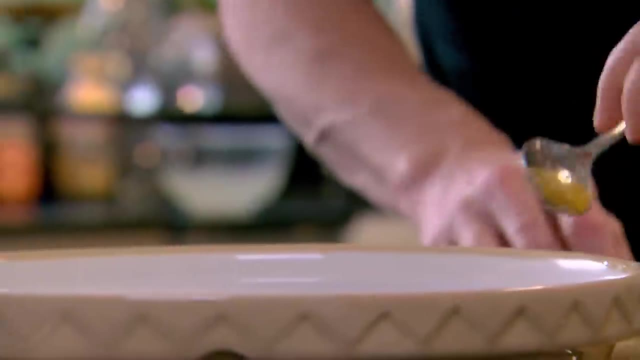 we'll either leave them whole, half or in quarter. What's that in there? Ginger? That's right, That's stem ginger. So we're going to use stem ginger and fresh ginger. Next, add your stem ginger. a little of the stem ginger syrup. 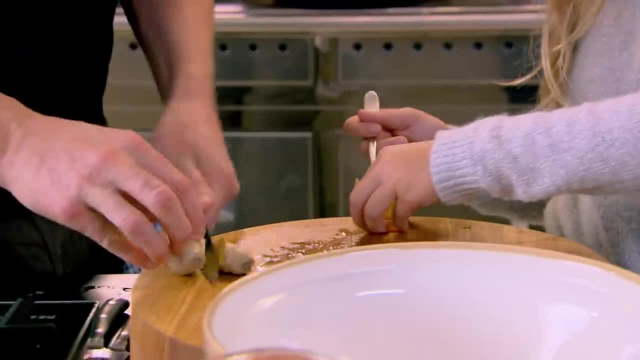 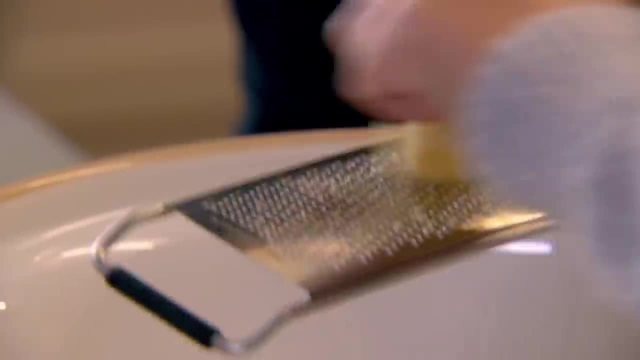 and some brown sugar to your quartered pears, OK, And then just grate some fresh ginger off you go. So it's a bit of a different one to grate this, because it doesn't really come through like the cheese. No, We're going to make that a little bit zesty. 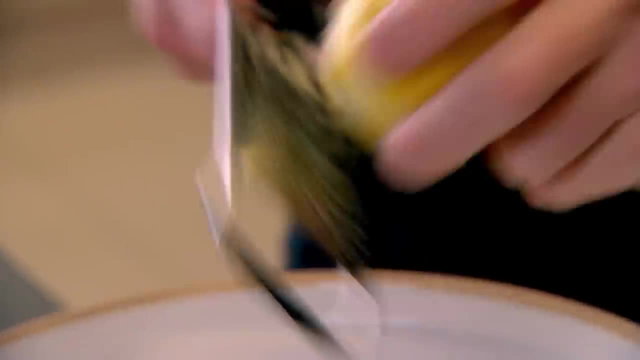 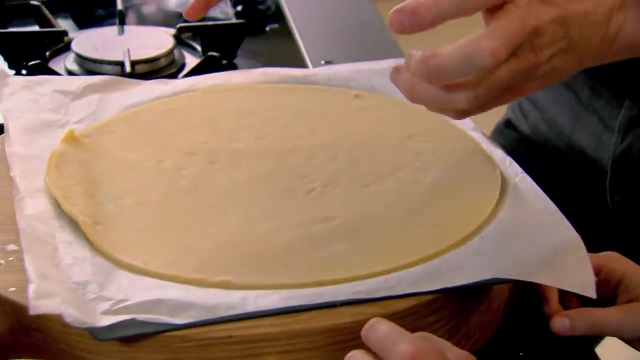 And now we've got some lemon zest, Some lemon zest in there, Right, what I want you to do now is give that a nice little mix. Now, this is a sweet pastry. You can buy this stuff or you can make it. 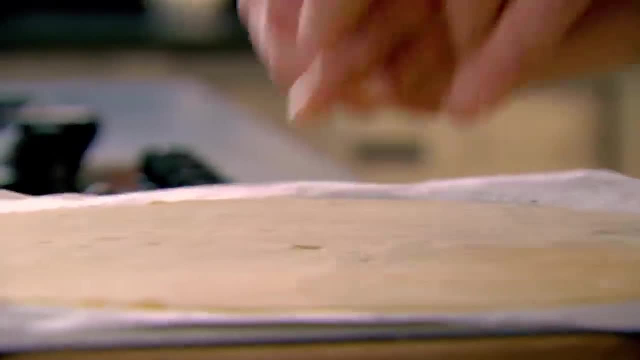 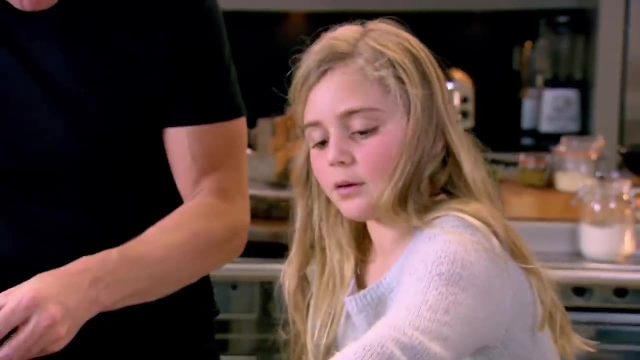 It's so easy to do. So give me your finger. That's my center point. I want you to get it. The pears go around like that in a really nice circle. It's difficult, isn't it, Because the pears keep on sliding all over the place. 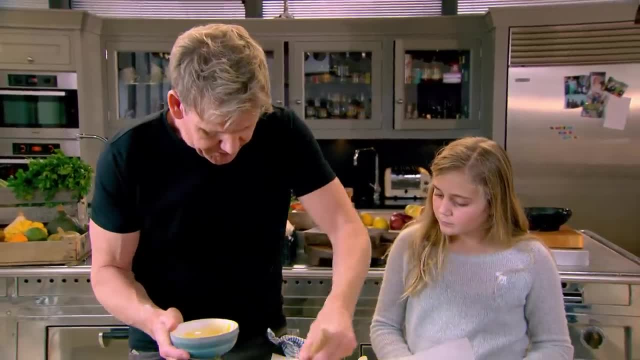 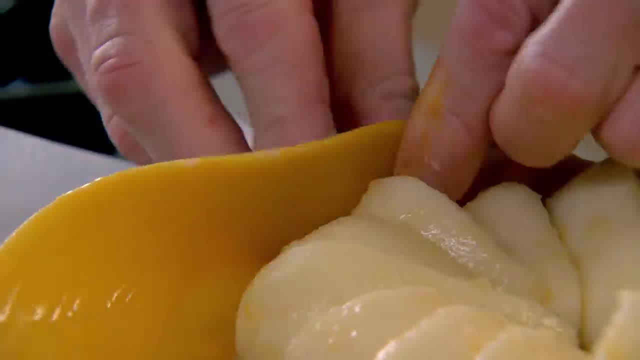 Yeah, We've got egg wash on the outside And I'm going to show you a little trick. So you lift that up. So is the egg wash acting like a bit of a glue, That's right. Crumple this with our finger and the pastry. 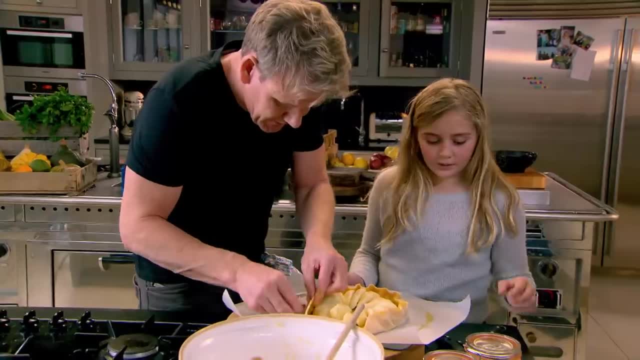 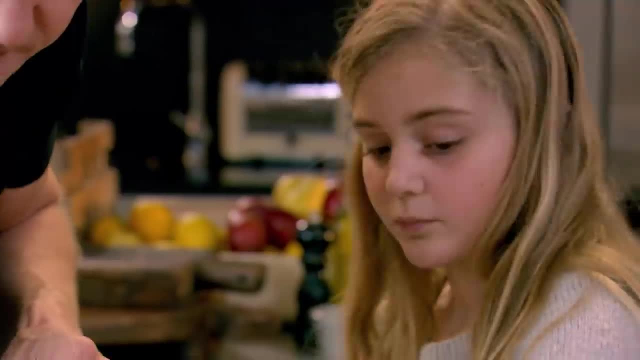 forms this nice little shelf like a little money bag. Are you going to do anything with the spare pears? Oh yeah, You start building that up. Then you see We've got the fresh ginger and those nice little bits of stem ginger. 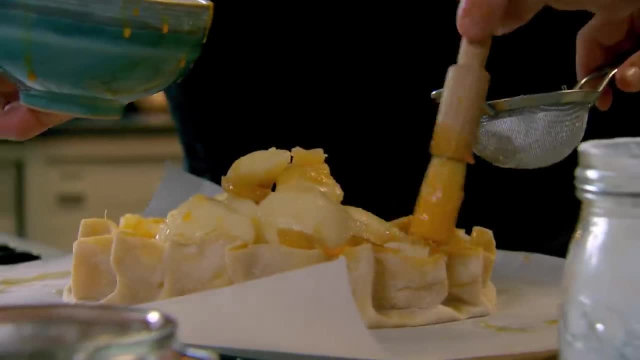 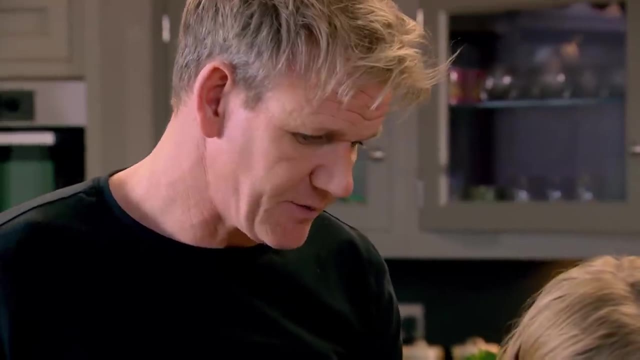 Let me go around, Meg, With your glue, With my glue, just on top. Tilly's last job is to give our tart a good dusting of icing sugar So that caramelizes it and colors the pears beautifully. It's a bit like snow. 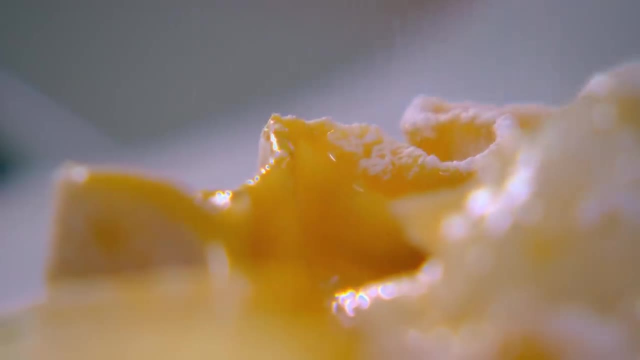 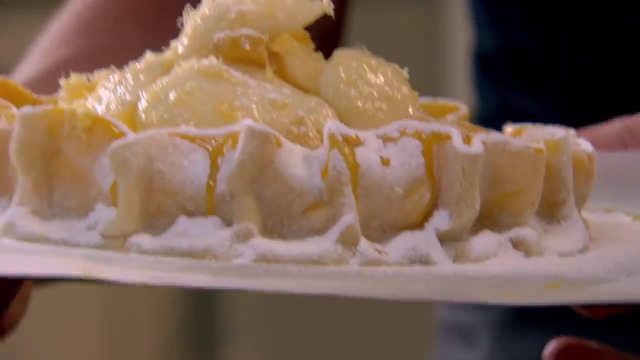 Isn't it? Now that glazes the pastry, So the pastry has this really nice shine on there as well. Finally, the lemon on top, And then put that there 180.. And into you. There she goes. Can you smell the beef? 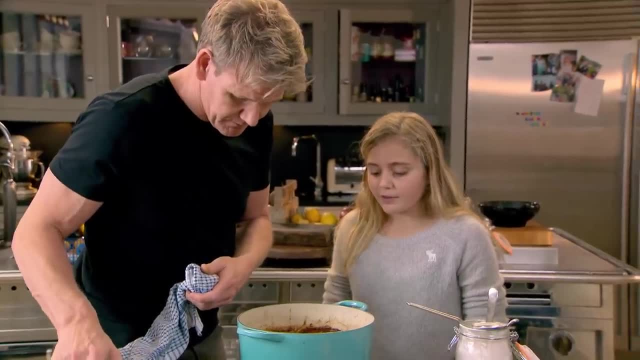 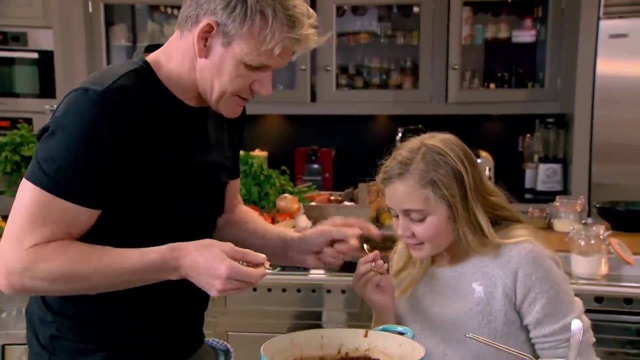 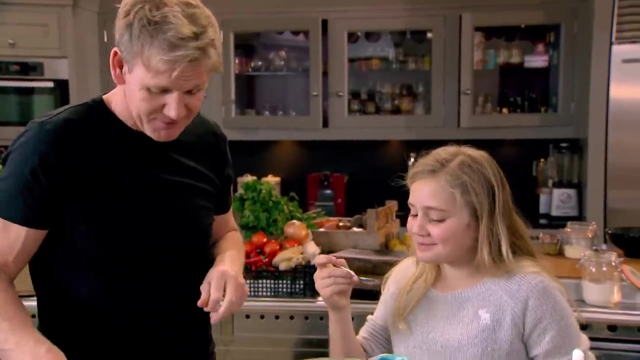 It smells delicious. Wow, it's even gone down a bit more, hasn't it? Look at that? I want you to. just I was hoping you'd ask: Just have a little taste. How's that taste? now Not loud anymore. 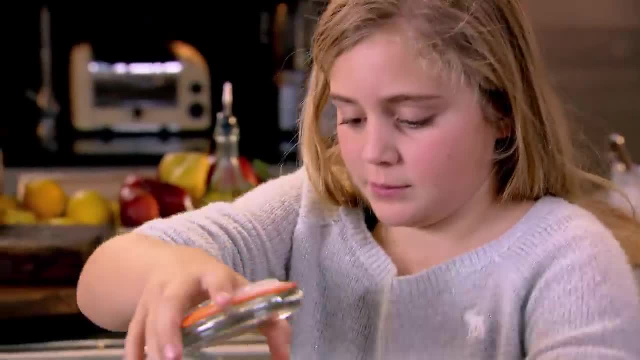 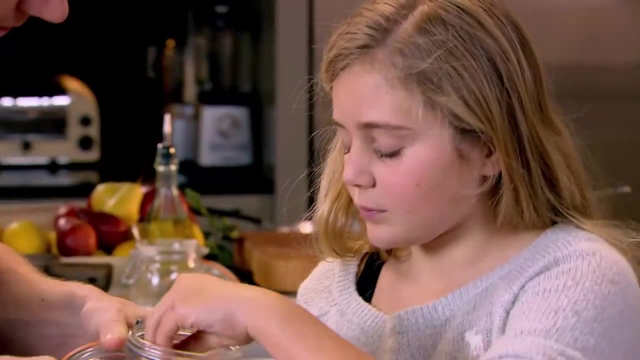 Dumpling time: Flour in. I'm using self-raising flour for a fluffy result, But if you like your dumplings hard, use plain flour. Next, the dumpling essential suet. That makes the dumplings nice and moist. 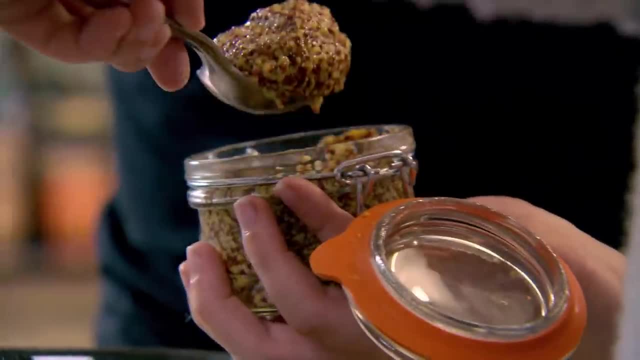 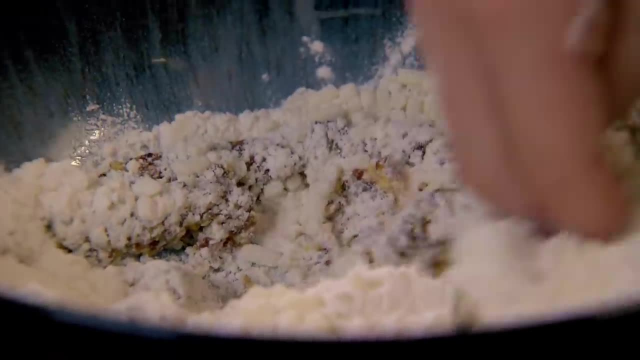 Thank you. Followed by a generous dollop of grain mustard, Two fingers Start rolling the fingers around And I've got a touch of warm water here. Your fingers are now a nice little whisk. Fingers are getting tired, Right. 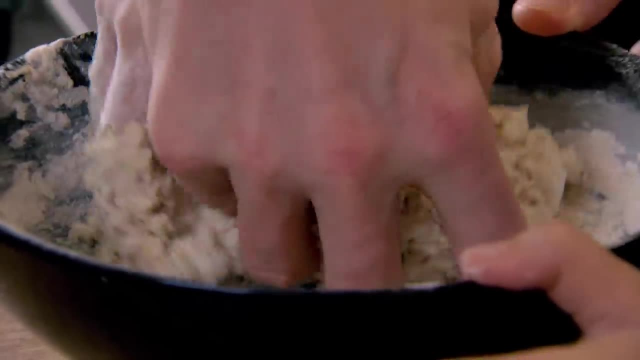 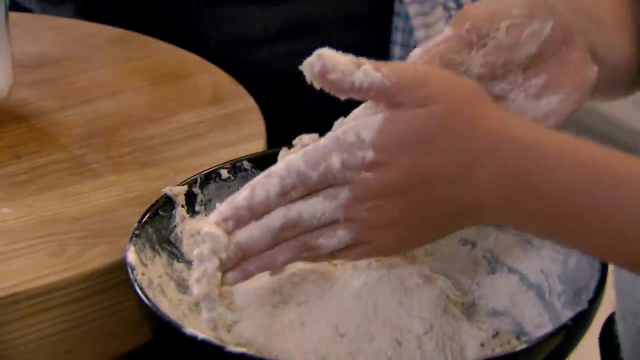 You've got some grain in there. Now you should bring all that dough together. I'll show you the best way to get that nice and clean. Sprinkles of flour on your hands. rub them together. All that will come off Nice. 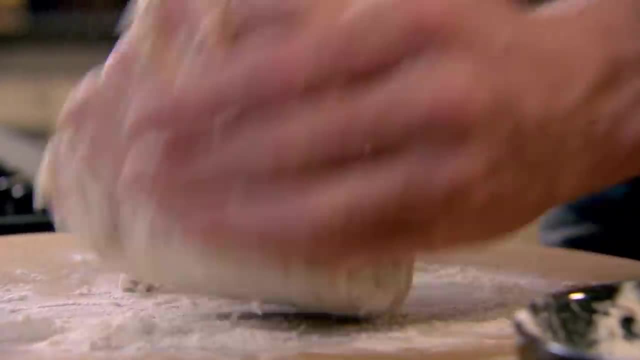 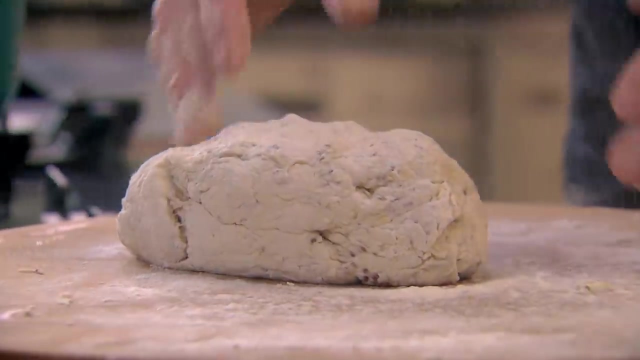 That's a good way, Isn't it? Now you've got this wonderful dumpling mixture. How squidgey is that? Ooh, A little flour on your hands. OK, Roll these lengthways, And then I want you to roll them like that in your hand. 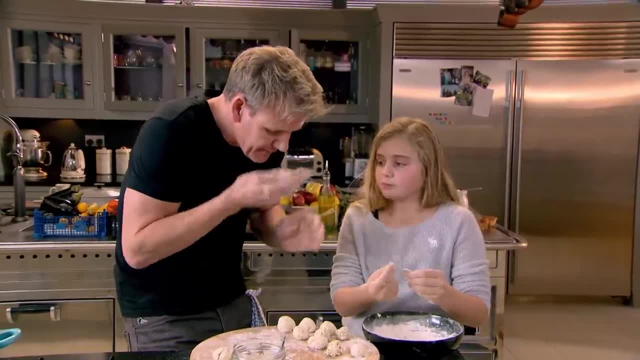 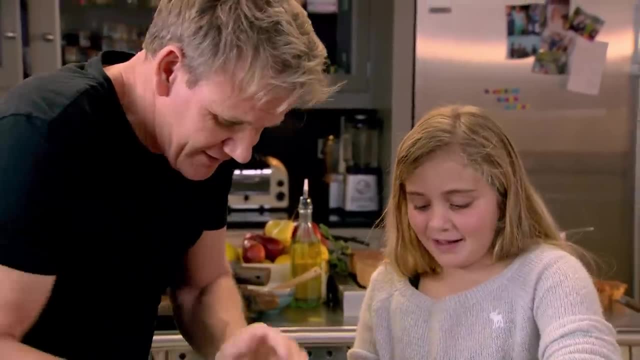 Off you go. Smell that mustard in there. Huh, Smell, Ooh. Come on, I'd never trust you with something like that, should I? Do you want to smell it? I'm beating you, Yes, please.